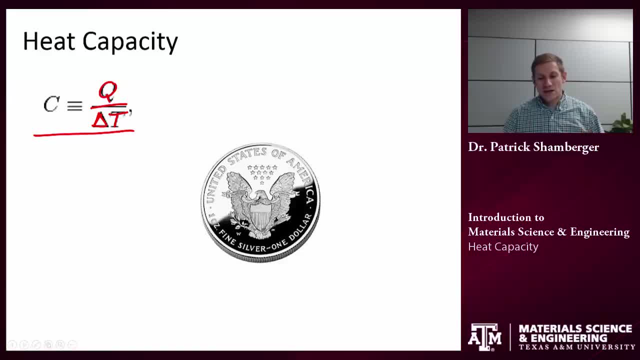 So usually I think about how much heat does it take to raise the temperature by one degree Kelvin, And we call that term the heat capacity. Oftentimes we would talk about a constant pressure or constant volume heat capacity dependent on the conditions of the energy. 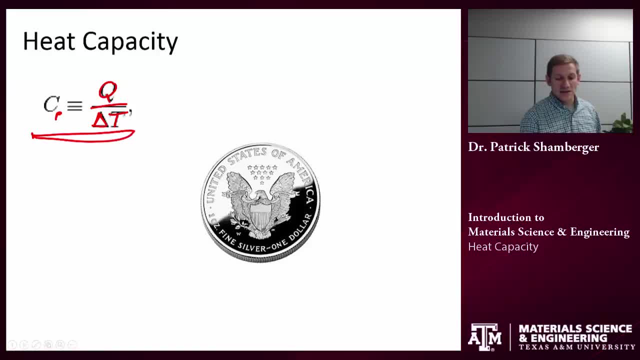 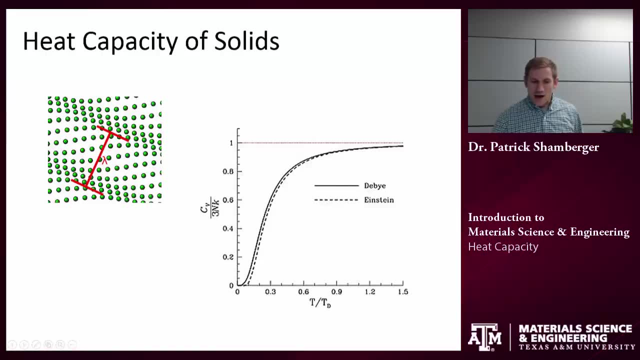 So the main thing I'm interested in is how much heat is the material in the experiment. Now, what is the heat capacity in a material? What difference does heat heat make in a material when it's in the room? And I'm interested in the difference between what the heat is and how much heat is being. 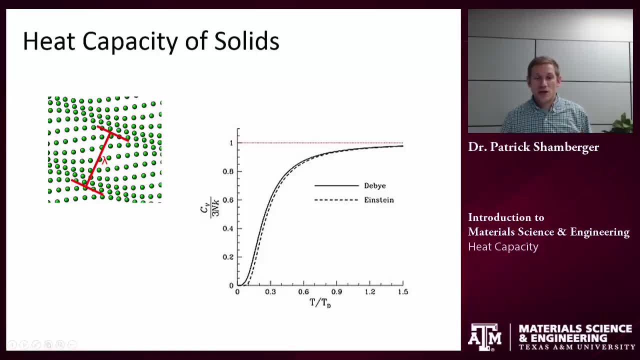 stored in that material. So the largest contribution to heat capacity is lattice vibrations. As I keep heating up a material, the lattice can vibrate more and more and in different directions, So I'll talk about that in just a moment. So we're going to look at the different variations. So what you can see in this reaction is the 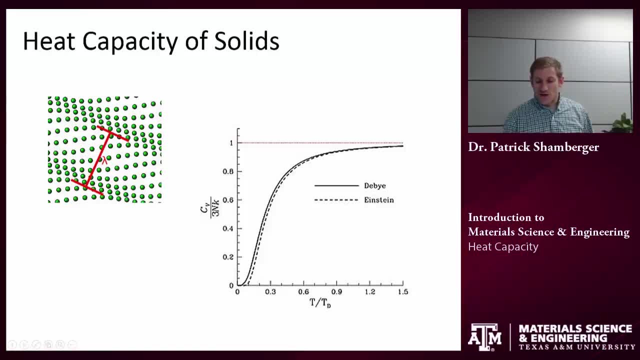 So this gives rise to a very interesting phenomenon, right? because if I think about a system at a very low temperature, if it's at a low enough temperature, then I don't have enough energy to access the different vibrational modes, right? 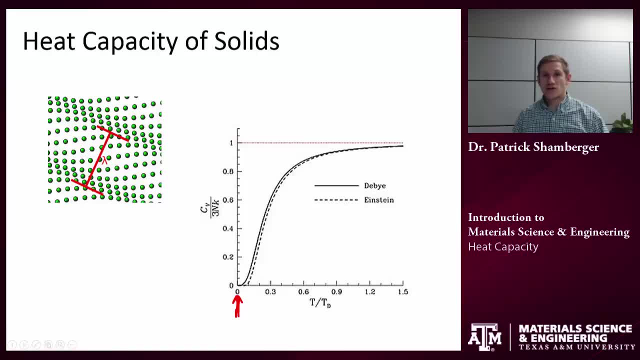 Phonons. we talked about phonons in a previous video but, just as a reminder, phonons are quantized lattice vibrations, so they each have some energy associated with them. So the material has to start warming up before I can access some of these different vibrations. 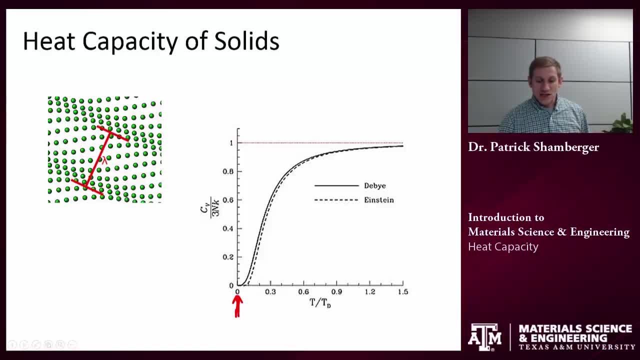 So, at very low temperatures, the heat capacity of materials always goes to zero, goes to a negligible amount, and that's because I don't have enough temperature to start accessing the different phonon modes, the different vibrational, the different vibrations that I can access. 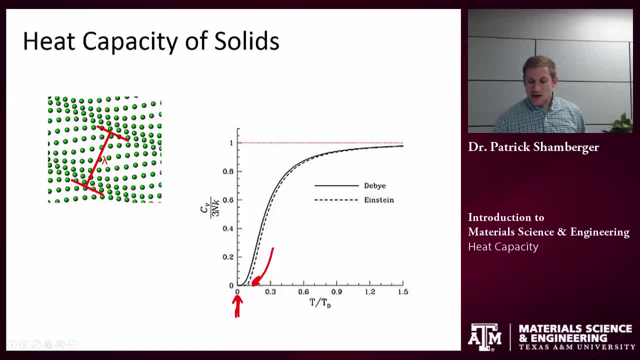 in a real material. As I continue heating a material up further and further, I'm going to start heating it up. At some point I'm going to be able to access all of these different vibrational states And so what you see in different materials. 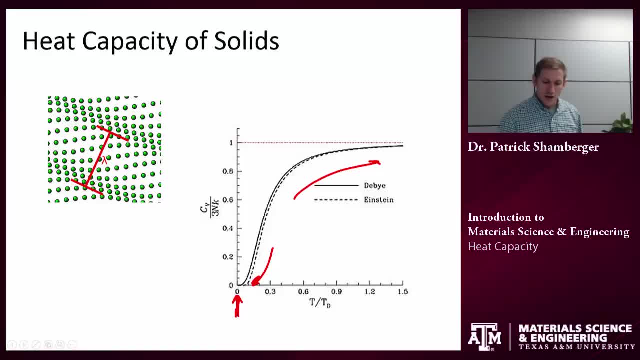 if we're only looking at the lattice contribution to heat capacity, all materials will asymptote out to the same value, And that value is given by 3NK or alternatively 3R. So R is the ideal gas constant, K is Boltzmann's. 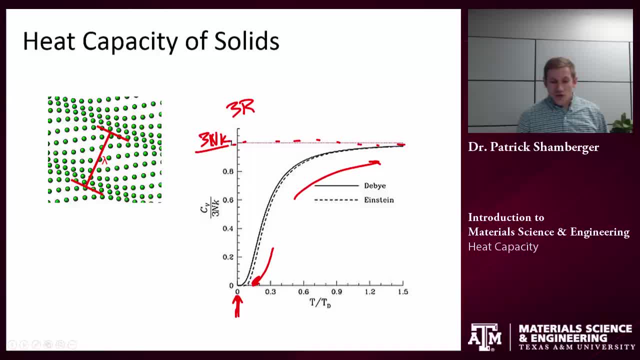 constant and N is Avogadro's number. So the heat capacity is ultimately a function of how many atoms are there in the material, And this is why different materials are going to have different heat capacities, because usually we think of a kilogram of a material. 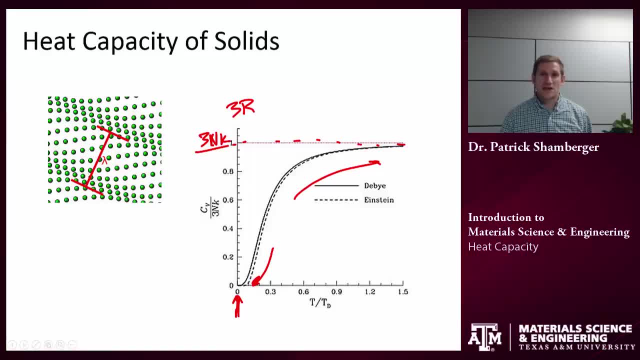 and we would give a specific heat capacity, so heat capacity per unit mass. In that case, one kilogram of lead is going to have a lot fewer atoms than one kilogram of aluminum, say. So they would have different specific heat capacities. 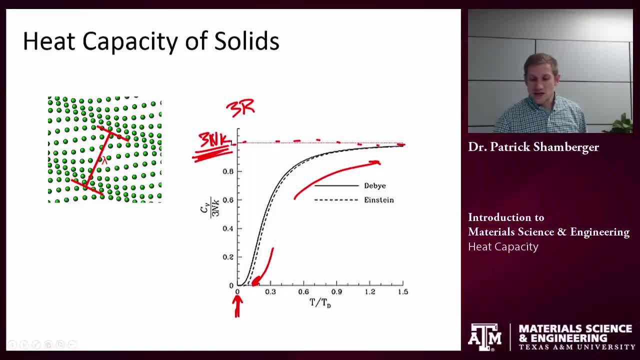 But on the atomic or on the molar basis. the heat capacity for all these substances is going to approximate 3R at high temperatures. So what do I mean by high temperatures? Well, each material has a different, what we call the Debye temperature. 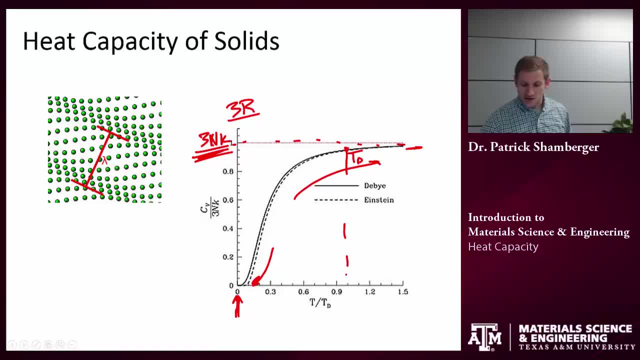 So the Debye temperature is a temperature it's right about here. it's given on one because I've normalized this axis here. But the Debye temperature is the temperature at which I'm able to access most of these vibrational modes. 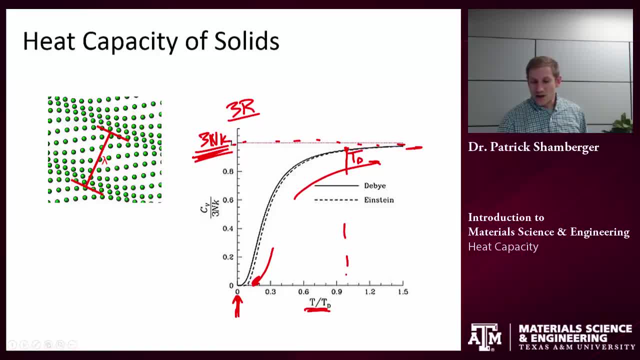 So by the time I get to the Debye temperature, the heat capacity is almost constant for all these different materials. So let's think about a different way to plot this graph. Instead of normalizing, let's just plot it on a traditional temperature scale. 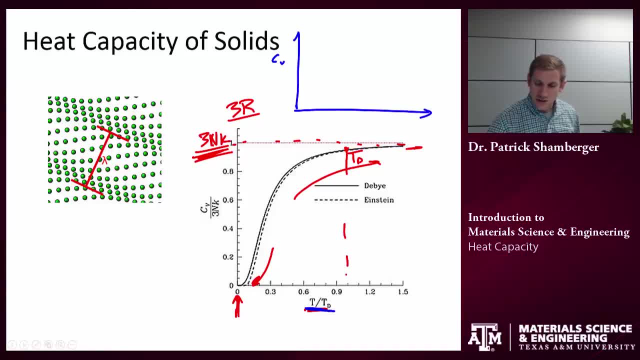 So if I'm plotting heat capacity versus temperature for a number of different materials, Some materials I would see a relatively low Debye temperature. So T sub D would be relatively low on this material. Another material: I might see a relatively higher. 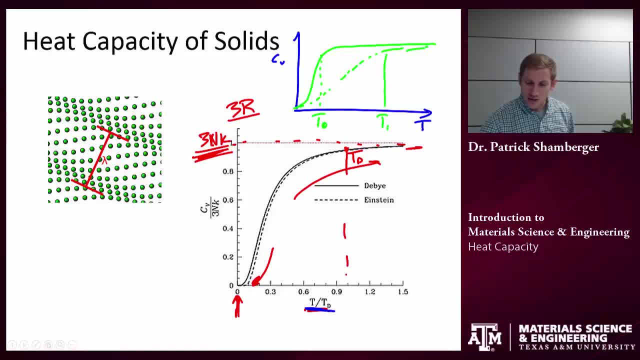 Debye temperature. So it's somewhere out here, But they're all asymptoting to the same value And if I collapse, if I renormalize by the Debye temperature, then I actually see quite good correspondence between different materials on this kind of a chart. 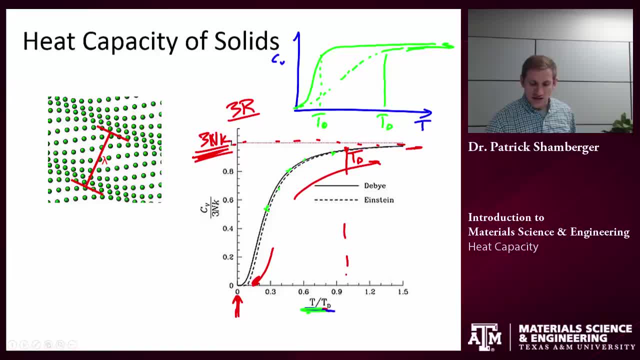 So I could plot it up and I could see metals and I could see semiconductors and I could see ionic materials, and they all would tend to follow this same universal curve. So it's really interesting, right.